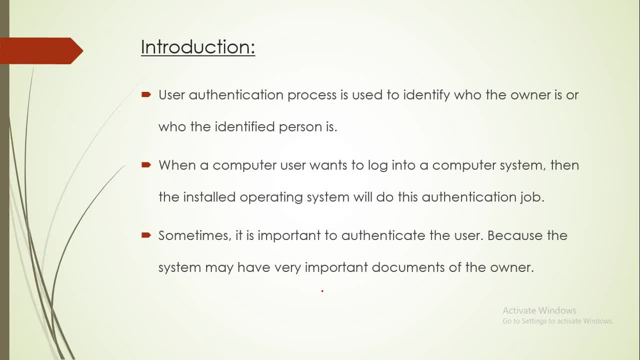 documents of the owner. So if I'm, if I'm the owner of my computer or system or my mobile phone, I may have, I or I have and I have stored many important documents in my computer system And if any user wants to access to my computer system, obviously he will get access to my documents also. So at that times it is very important to authenticate the user or to identify or identification of user at that time. 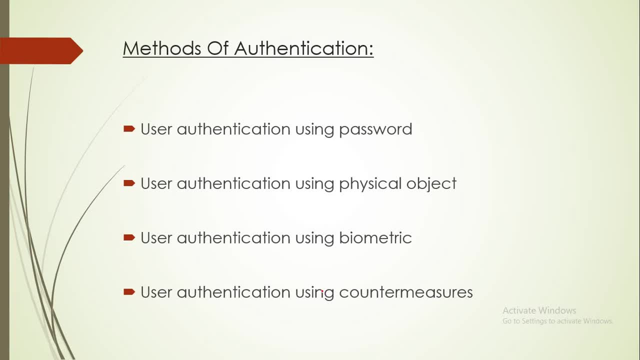 Next is methods of authentication, So the we can authenticate a user or the operating system will authenticate a user in the following methods, that is, by by using the passwords, passwords- or in the computer systems we will use password, and in mobile phones we will use password and patterns or any other means of application that is, using physical object. physical object. 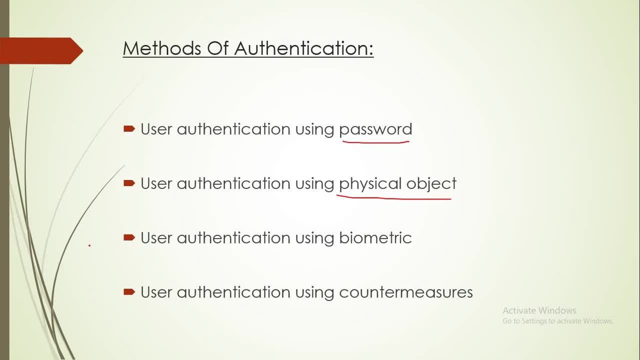 So authentication is done in case of ATMs. So if we want to access our account info or if we want to withdraw money, we need to use the ATM card with magnetic tape. all the information of our all the information of our account will be stored in that magnetic tape And that card is in that case. that card is known as the physical object. So by using that also we can authenticate ourselves, and using that we can authenticate ourselves. 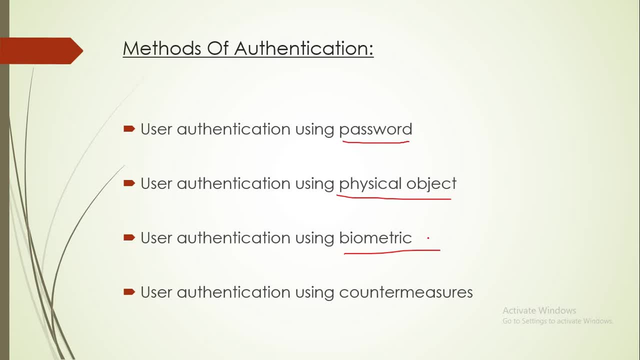 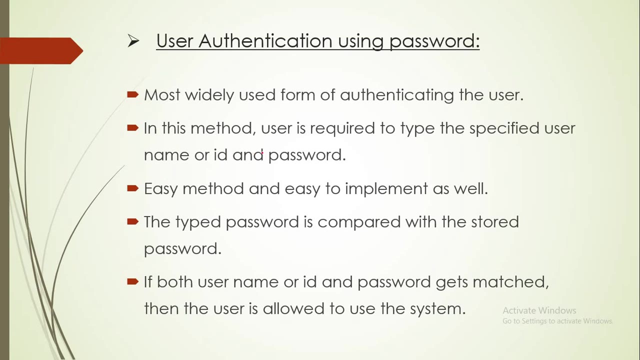 Next is biometric using biometric means- using fingerprints or retina like that, And user authentication using countermeasures and other countermeasures except this password, physical object methods and biometric methods. Next is user authentication using password. So how can we authenticate a user or identify the user using passwords, That is, password. Password authentication is most widely used form of authenticating the user. 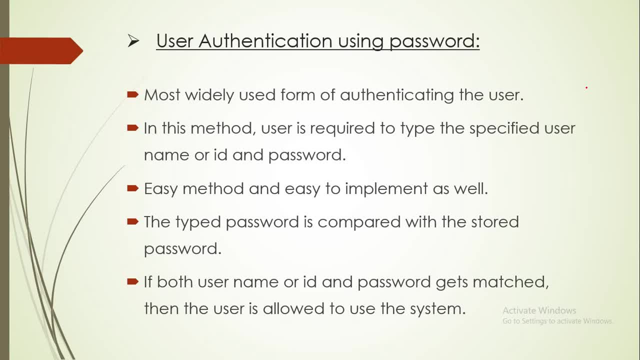 So this is most widely used and almost everywhere you can see passwords like while using the, while using your Facebook account or while logging into a mobile or while accessing a specific application in the mobile or or logging in into the computer system. At that time we will make use of passwords And in this method user is required to type the specified username or ID and the password. The user has to make use of the password. 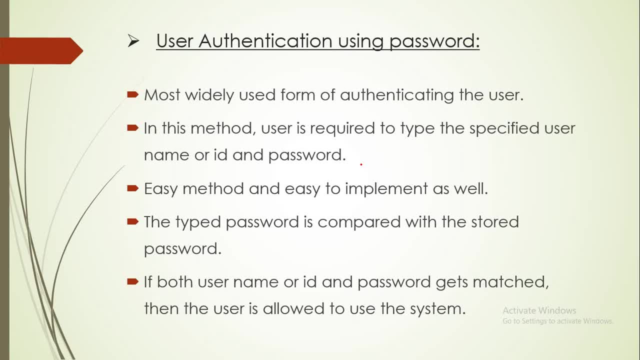 While doing that also, a user can mention the intended, intended or specific username or ID and password given to him, And this is the easy method and easy to implement as well. This is the easiest method. Almost we can see everywhere the password authentication method and it is easy to implement as well. The typed password is compared with the stored password, So the best example for this is while logging in into a computer system. 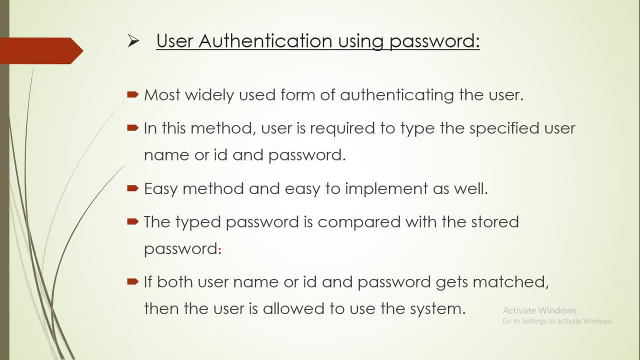 So, while setting up a website, up the OAS, we will, we will also set up the security settings, so where. so at that time we will give some password, so and that password will be stored by stored in operating system. operating system will take care of all those things. that password will be stored in the database. 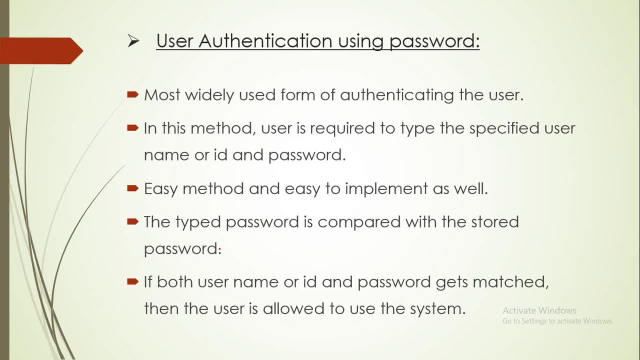 so when you when again when logging into the system, if you type that password, the typed password and the password that is stored in the database will be compared. so if that matches, the user is allowed to use the computer system, or else it will show the password is wrong, or? 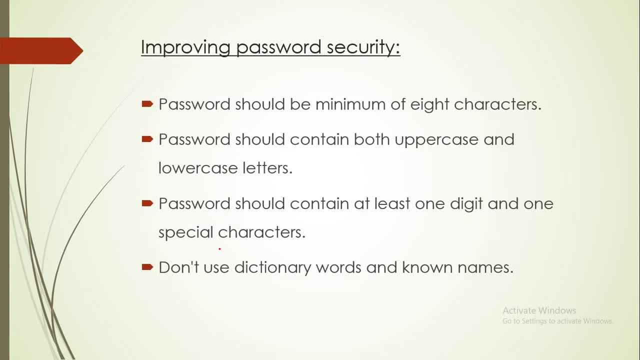 you or the user cannot log into the system. next is: how can we improve the password security? so, even though we have kept the security, password security for our documents or the for our whole system, at that times also hackers or malicious viruses can hack that. so at that time, how can we improve the password security and what? 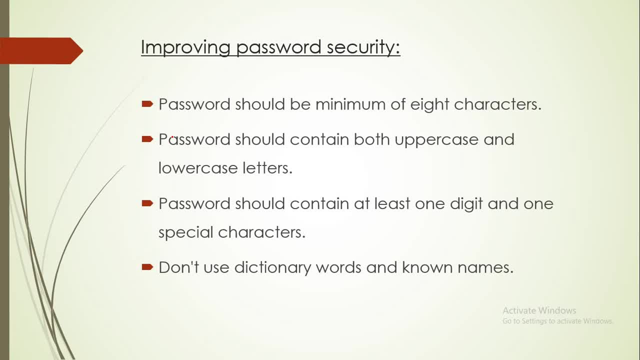 measures can be taken to improve our password. security means the password should be minimum of eight characters. the password should be: the password should not be so less in length such that the hacker can easily identify or easily recognize the combination of your characters. so the password should be actually minimum of eight characters. 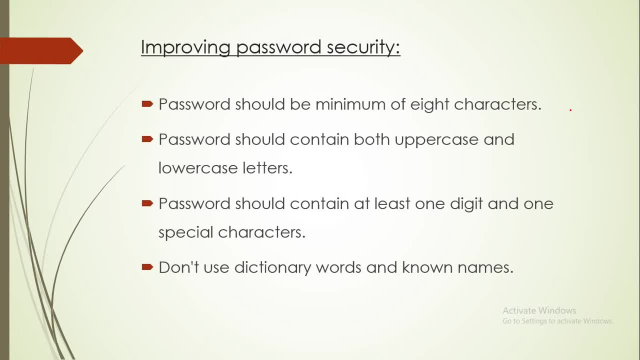 and maximum you can have in a number of characters in your password and it should contain both uppercase and lowercase letters. so if we, if we set our password using only lowercase and if the hacker gets any clue of that, he can easily, he can easily- hack our system and steal our documents. so